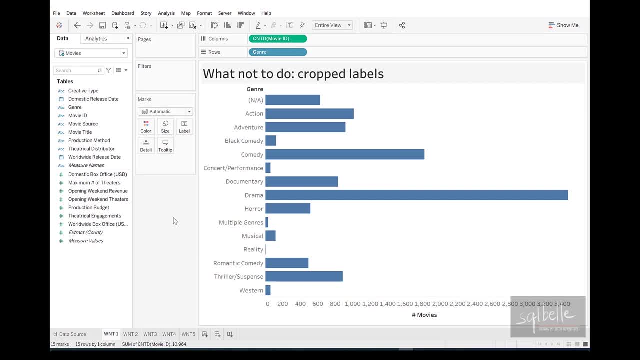 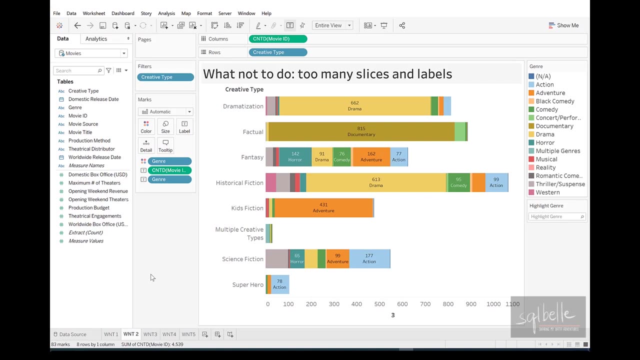 swap the rows and the columns With a horizontal bar graph. it gives us the ability to play around with the width of the label without sacrificing the value of the bars. Use case number two: too many slices and labels. I've seen this a lot and actually the questions. 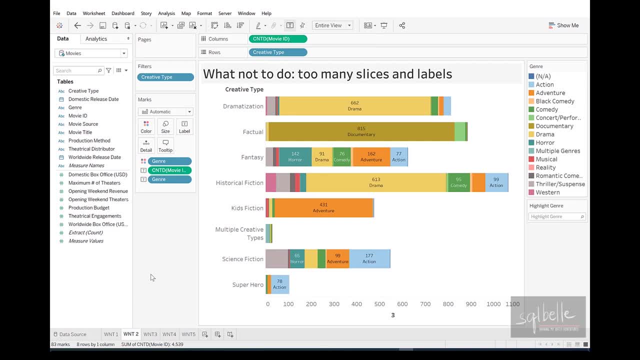 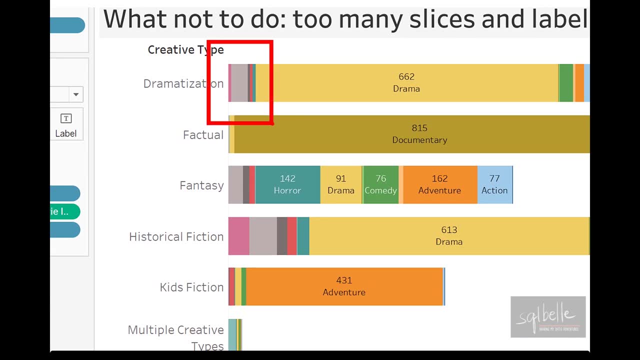 that I get with this type of chart is: well, you know, we don't see the labels for some of these areas that have really small slices. Is there a way for us to force it Technically? yes, Tableau will allow you to have overlapping marks. So when we go to label, 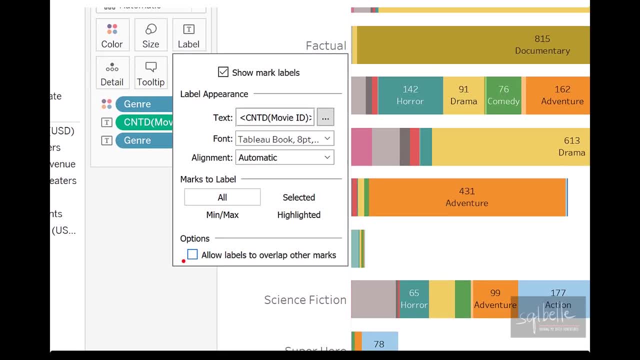 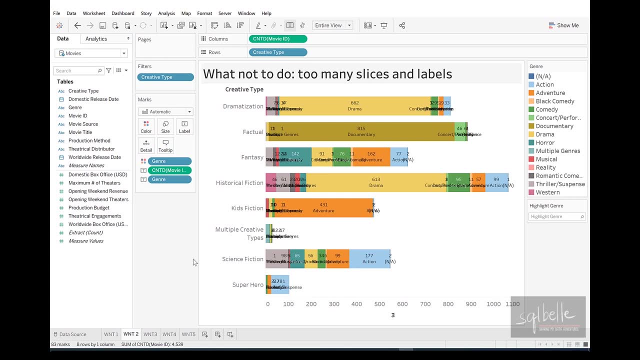 you can click on this option to allow labels to overlap other marks And once we select that, this is what we get. I don't think that's a solution, but that's a yes answer to the previous question. So right now, what we want to do is: well, what is the best way for us to? 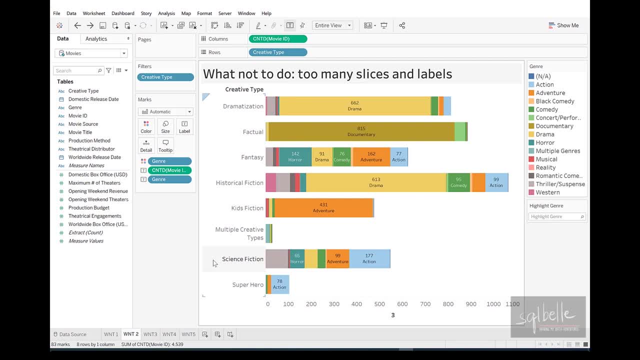 move forward if you have too many slices and too many labels. Right now we have actually too many colors, So first thing to consider is: is there a way for us to slice it up, not using color? That's one option. Another option in terms of the labeling piece is: we may not. 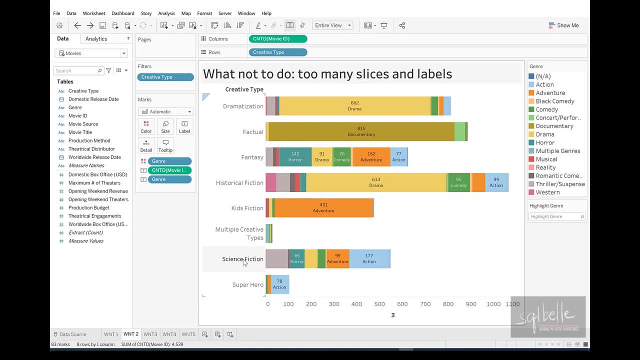 necessarily have to show all the labels, all the values right away. So in a tool like Tableau you can have some interactivity around it. So, for example, we can choose to show the label on certain actions, So maybe when it's highlighted. 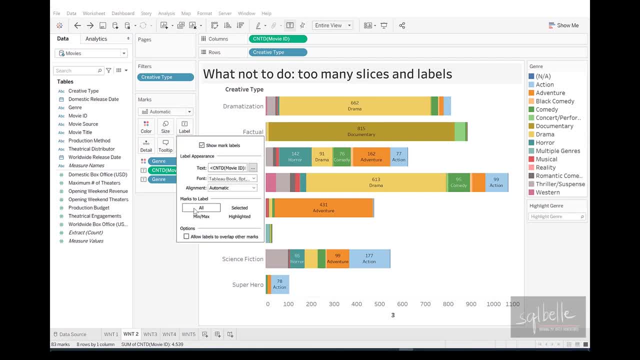 So when we click on label, instead of showing all right away we can simply say when it's highlighted, And then we can also just show the highlighter feature. So I've already turned that highlighter feature on, but you can find it from your pill. that is located in color. So in here. 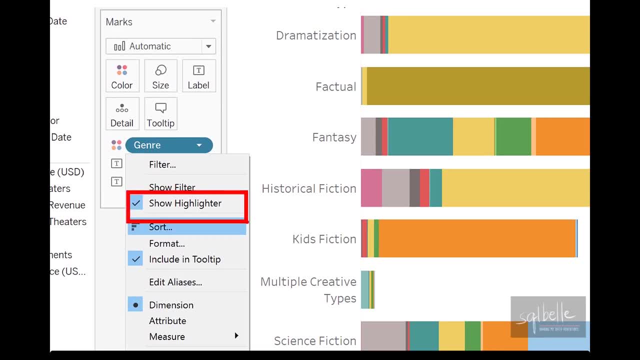 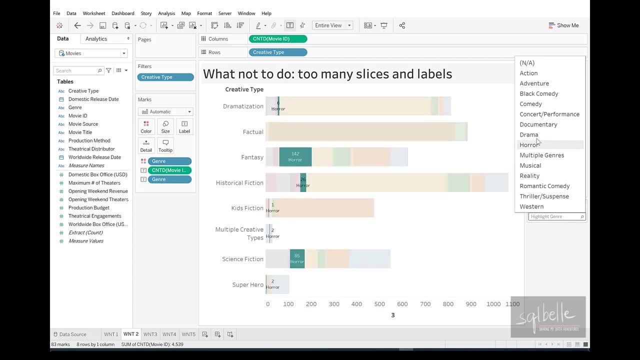 it's that show highlighter. It's actually this one right there, And what this does is now the data will be on demand. It's still going to be a little bit confusing, but at least it's clear what those values are. They don't overlap. 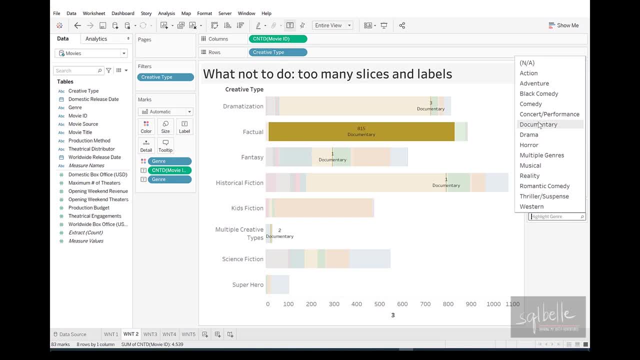 and overwhelm all the other labels from all the other values And in some ways this is again. this allows for more engagement with your, with your audience, with your end user. They hover around, they look at the values and at least they're able to see very clearly what those tables are. 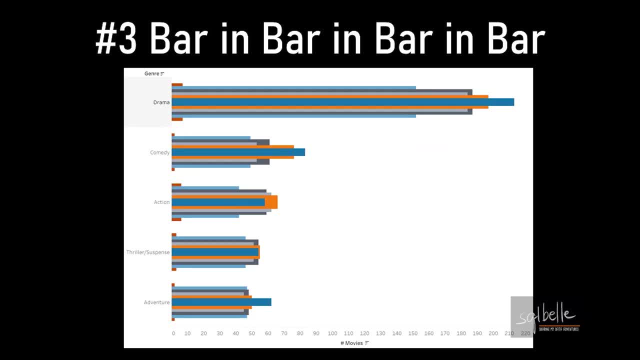 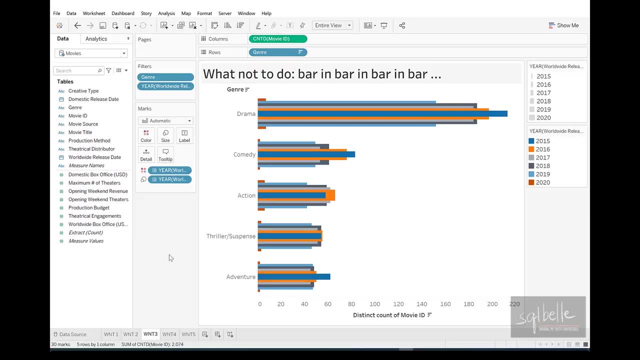 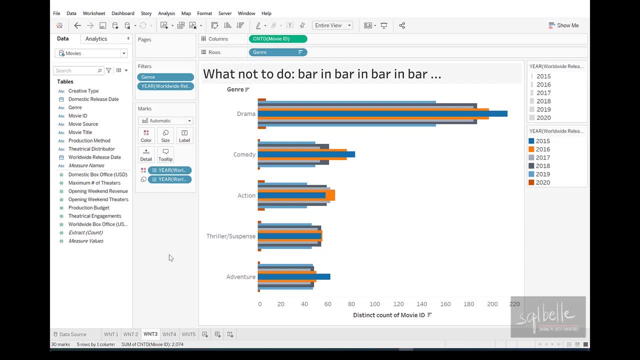 together. So instead of having two bars side by side, what you do is you superimpose one bar on top of the other and you vary the color and the width of that bar. So it's a very compact way to compare two measures together. But if you wanted to compare more than two measures- and you may- 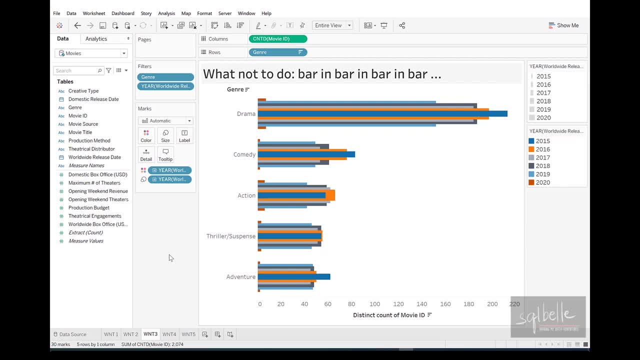 decide to do it this way. well, it looks fancy, It looks like a tower or a structure or a building, but it's very confusing. There's too much going on and it's quite overwhelming. The message isn't clear, The numbers aren't very clear, So my recommendation is, if you can keep it to just 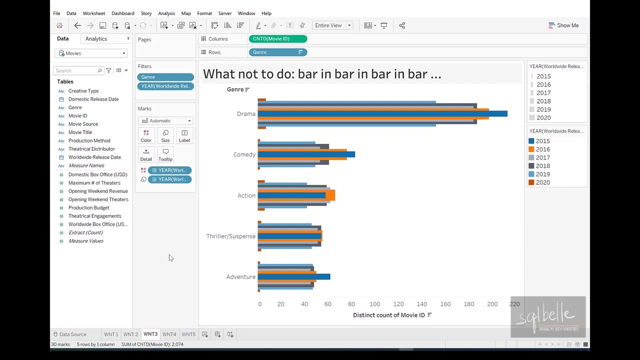 two measures if you can, But if it's really important for you to show six different years, this may not be the type of chart you're going to be using. So, again, I'm going to show you an example of how you could go around it. I'm not necessarily 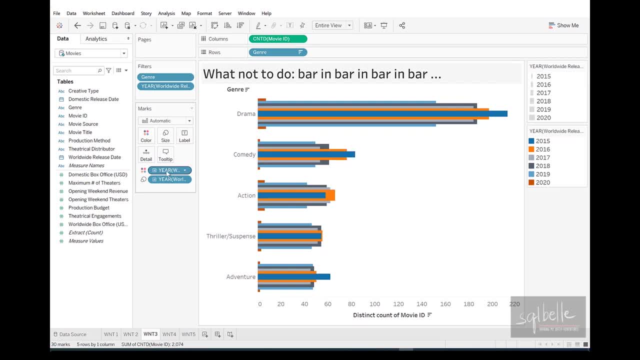 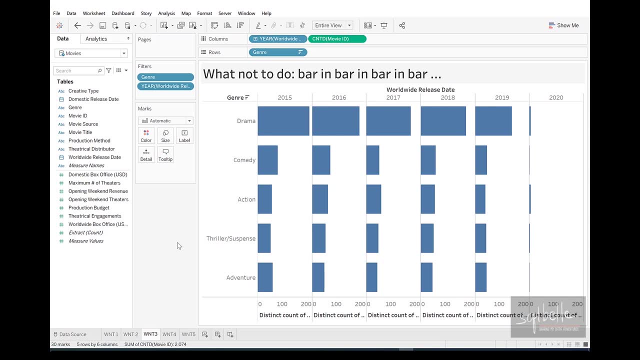 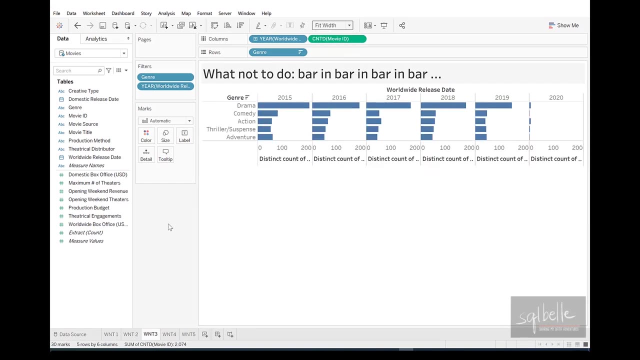 saying that this is how you should do it. but we could decide to just move year onto your columns and allow for the comparison of the different bars kind of independently. This might look like a more boring chart, but it is still a cleaner chart. It's still a clearer chart. So this is 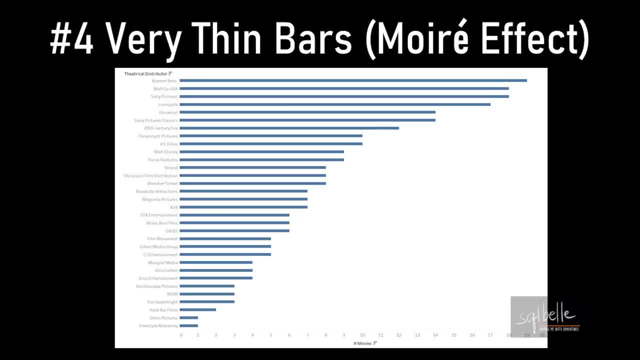 something to consider. Use case number four: very thin bars. So here's my challenge: Stare at the screen for about five seconds And this is probably very distracting for you. It's like the lines are changing, they're glimmering and you're going to have to look away because at some point this is very 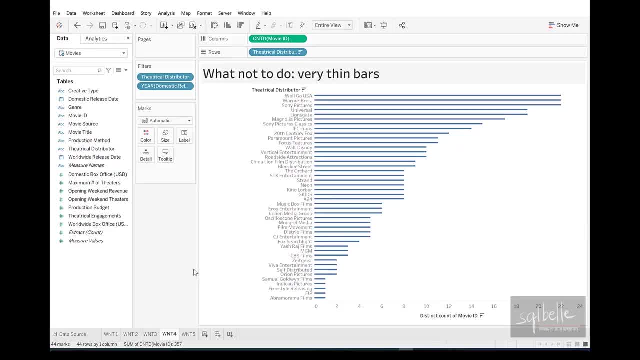 either hypnotizing or really just disturbing, But what this is is what we call a moiré effect. A moiré effect is when there is a perception of vibration, and it's also very distracting. So when we encounter this, first things first, let's not alter the width, So in this case, maybe we just need to adjust it. 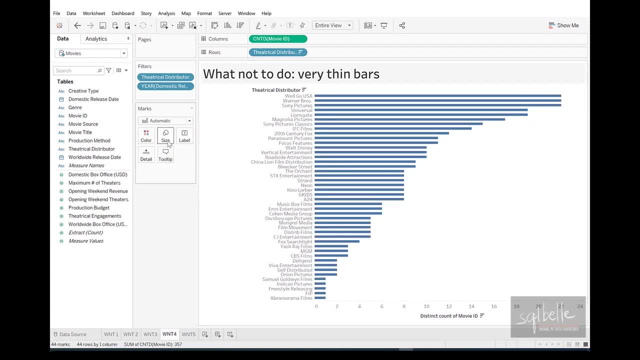 to a normal size or whatever the usual size is, So as long as it's not very thin. But the other thing to consider looking at this chart is there's too many data points that we are showing up front. What is the value that we are showing? 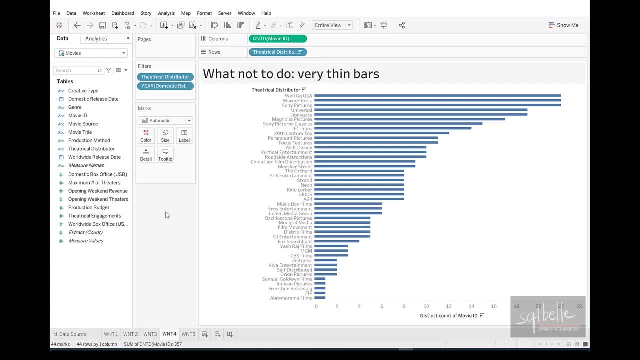 Right now. the challenge is: sometimes we are asked to show all the data right away, And sometimes it's just because we are so accustomed to seeing all the data, But this is an opportunity to see which of these data points are most valuable. What is it important to show right away? Maybe it's 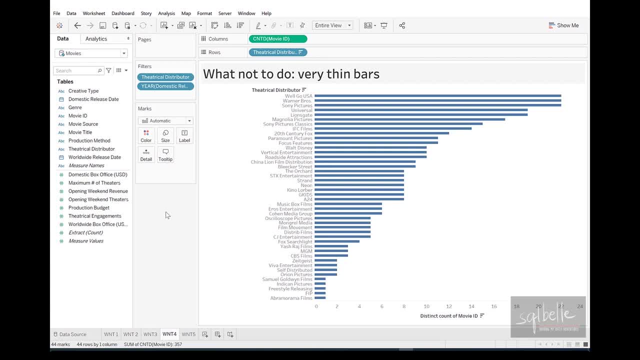 just the top five or the bottom five, or the top five and bottom five. That's still better than showing 50 different data points that people will have to scan through and they have to figure out What if this is of value to them when they're making their decisions. 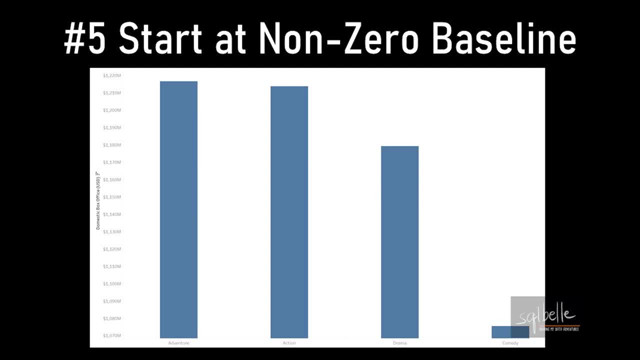 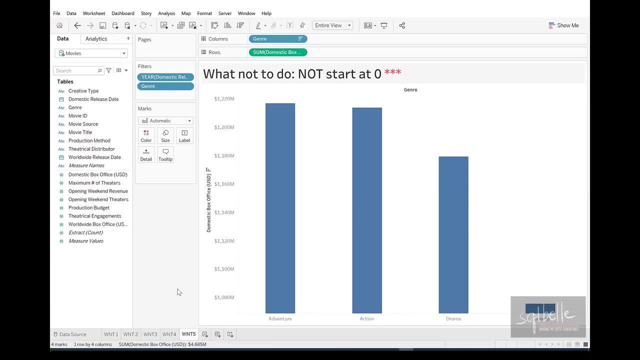 Use case number five: what not to do? Not start at a zero scale. That's a double negative. I don't think that was very clear, But notice, in here you have three asterisks. I put three asterisks in the title And it's because there are cases where it may be okay to start at a non-zero. 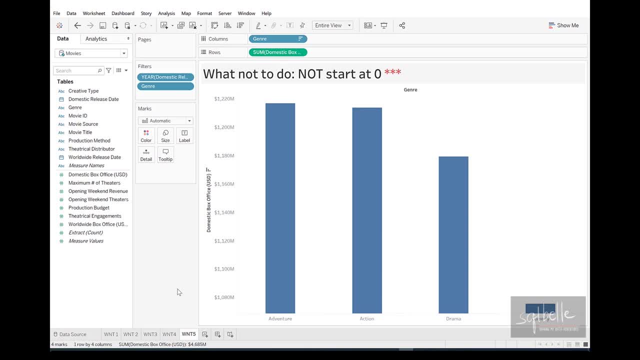 baseline And we'll get to that. But right now, at first glance pre-attentive attributes, what we see is we have a tall bar, a tall bar, a slightly tall bar and a very short bar. So in this case, in this particular chart, 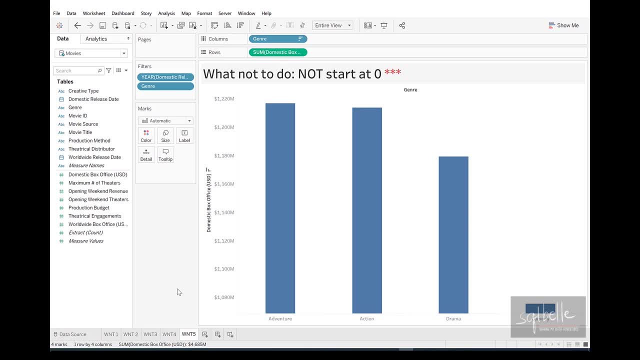 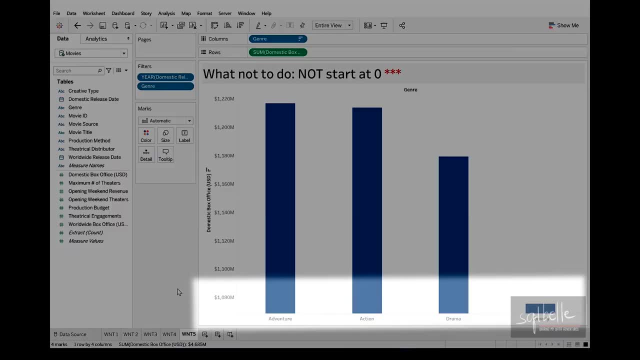 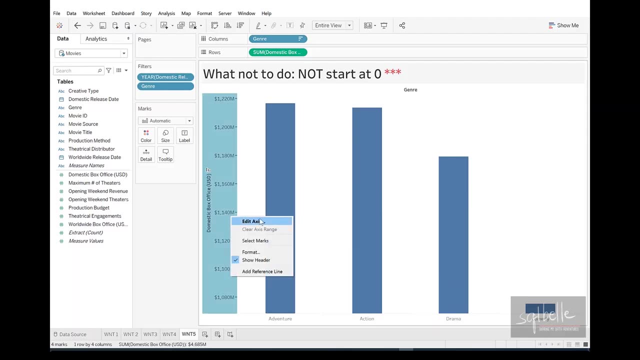 it looks like comedy is not making any money at all, But this is very misleading Because when we take a look at the scale, it starts from about a billion. It did make money In here. the effects are exaggerated because we did not start at zero. So what we could do is we can.